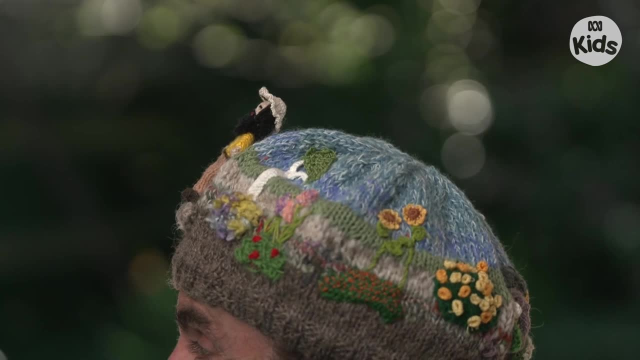 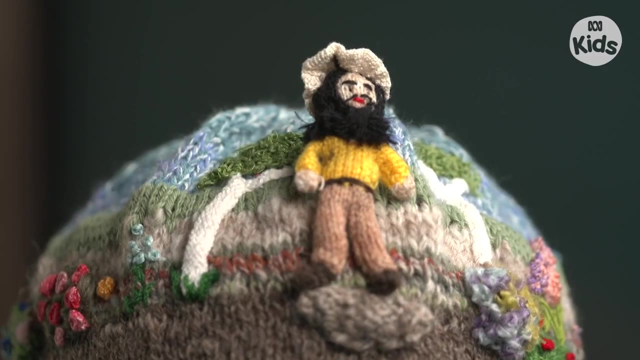 This is a magical garden, And look, the lady that made this is a woman. She was 93 years old, And that's you, Yeah. So what do you reckon? I think it would be good if we had two Custers working on the project. 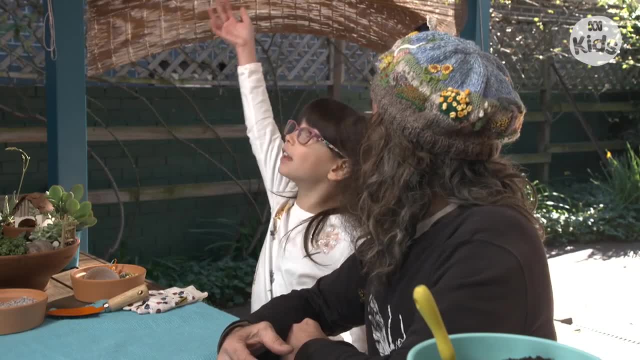 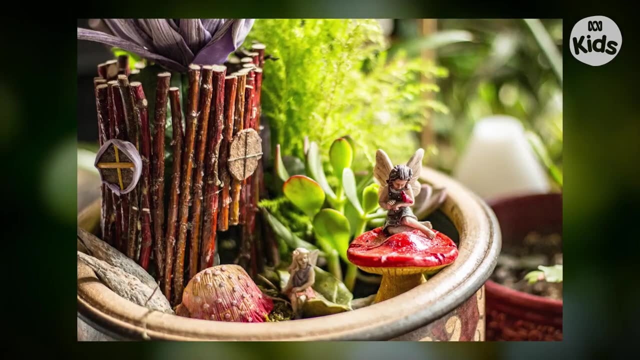 And one Kayleigh, Custer number one, Custer number two And one Kayleigh. To make a magic garden, you first need a pot. You can actually use four types of pots. That can be a broken pot or an unused fish tank. 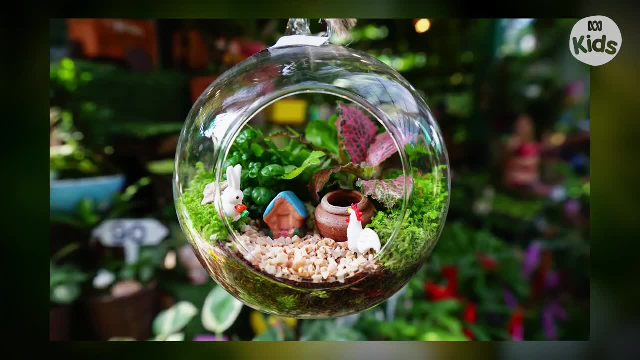 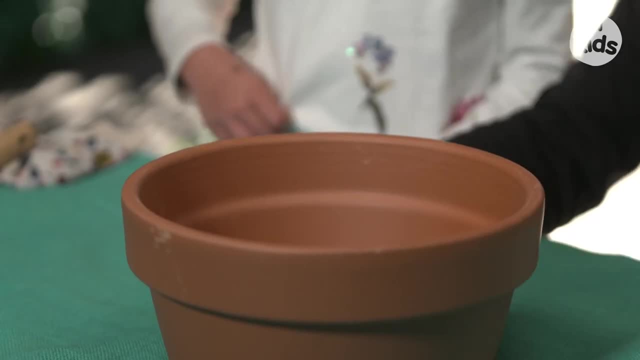 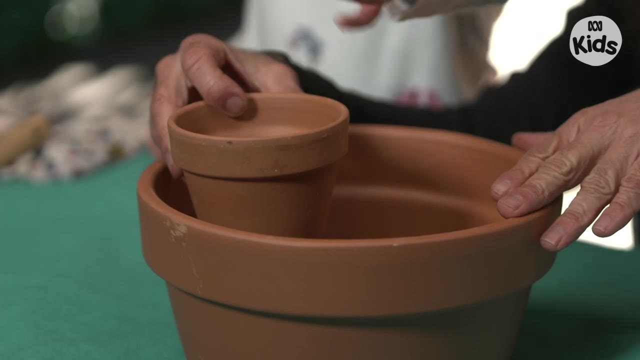 Or even an old teapot or saucepan, And then you can use other pots so that you can raise things up, So you can put a house in there. But if we want to make a fairy garden, don't we need plants to make a fairy garden? 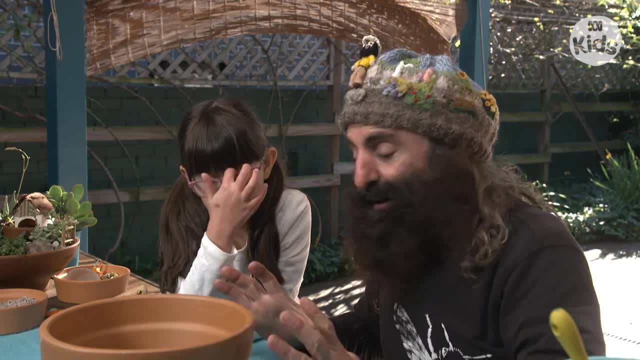 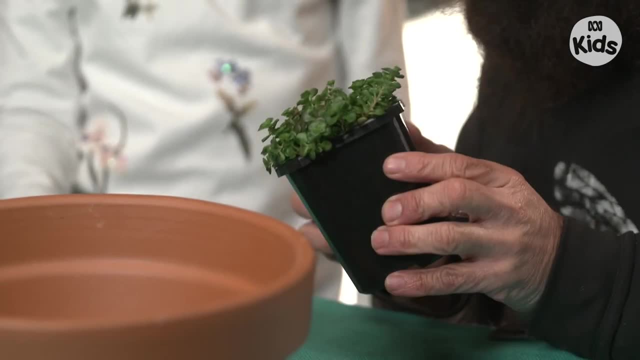 So what do we have to make plants? Okay now, the good thing about making a magic little garden is that you can use plants to get the effect that you want. So this succulent, which grows very low, can be like a ground cover. 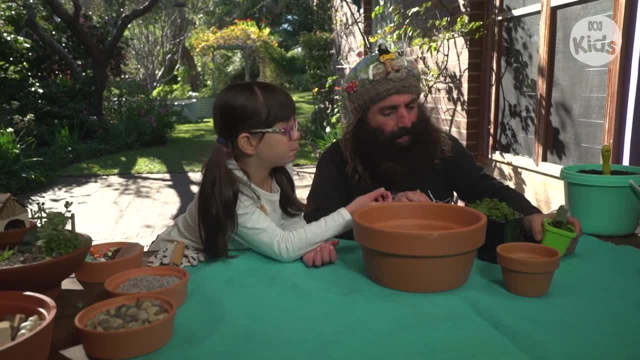 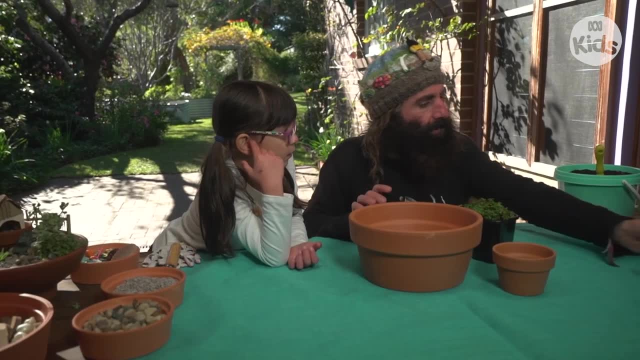 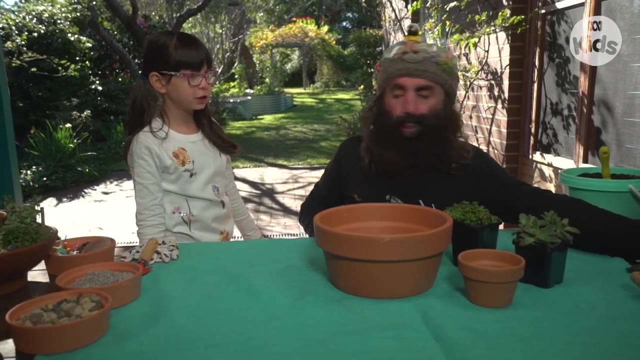 And it could be like a little place that you can add some bugs on top, Exactly, And that's like a nice feature because that sticks up. And then this one is a lot taller, so it's more like a tree. You can put the tall ones at the back so you can actually see the tall ones. 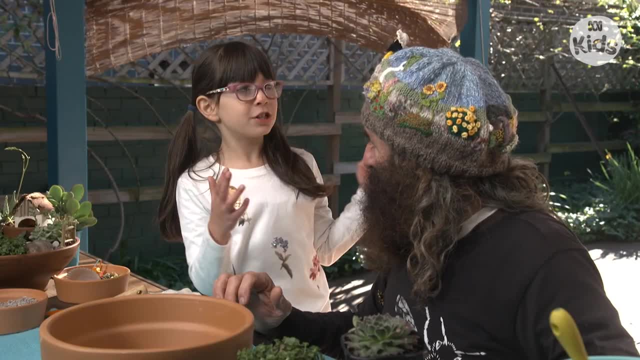 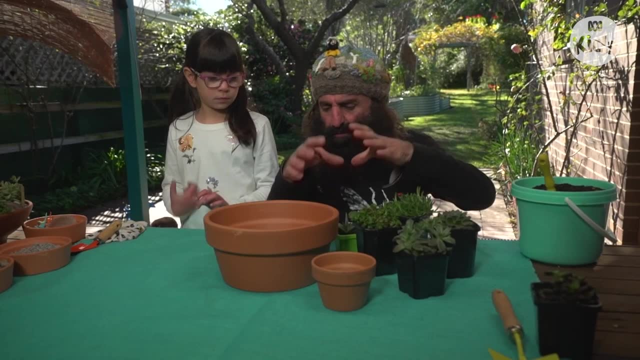 Because if you put the short ones at the back and the tall ones up front, how can you see the big, tall ones Exactly? All of these succulents are perfect because we can break them up into individuals or keep them as a clump. 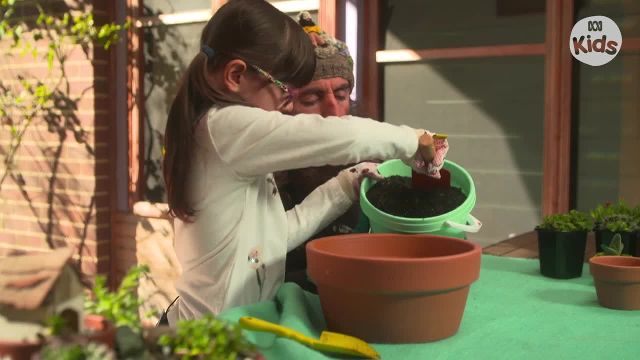 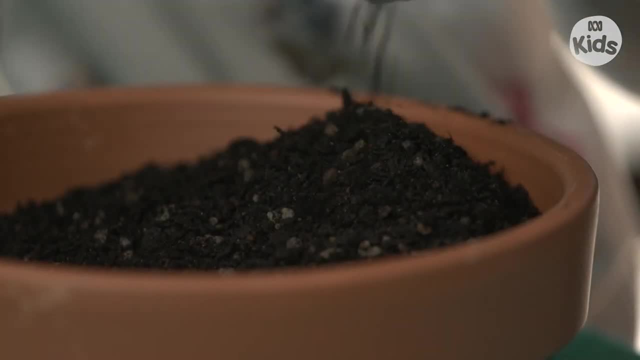 The next step is to put it in our potting mix, Because I'm planting succulents, I'm using a free-draining cactus and succulent mix. Oh, good job. You want it not to be too low and you don't want it to be too high. 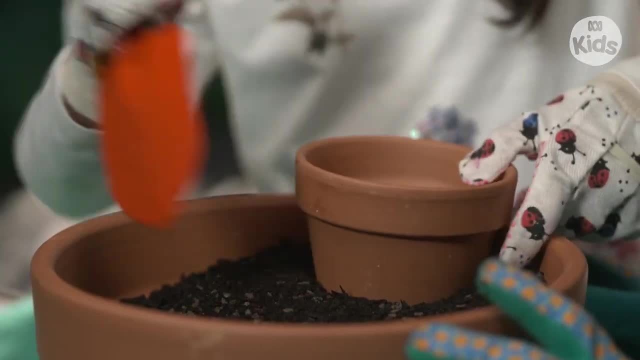 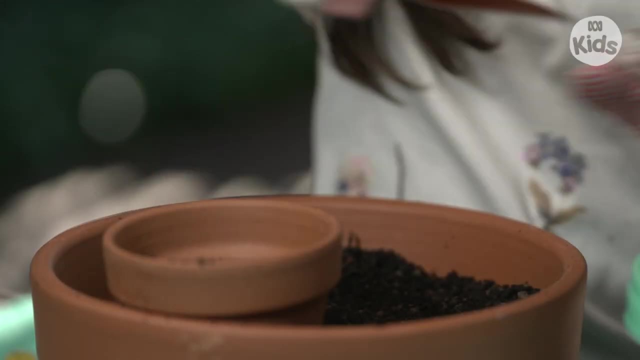 You want it to be perfect, so it's level like this: Put the smaller pot on top, settling it down into the soil to keep it stable. Fill in the little hole inside. Now the fun bit starts. Okay, here we have a house. 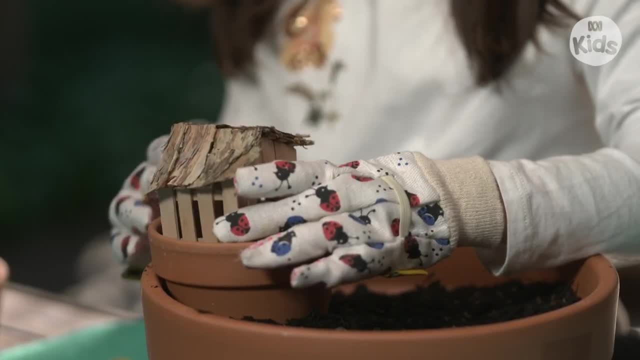 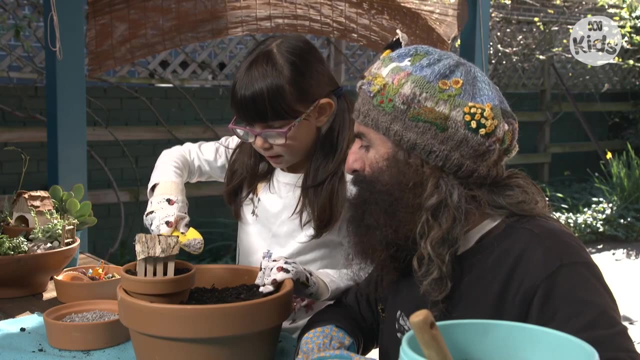 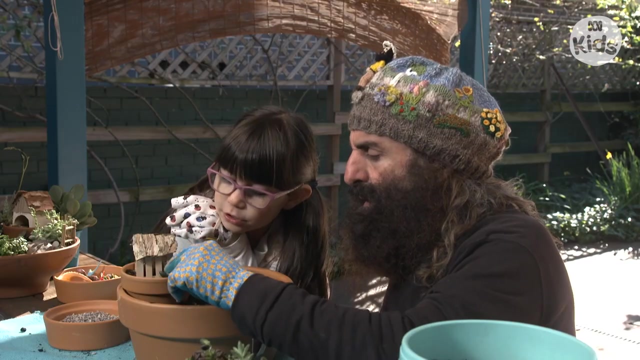 We made it, so it's quite nice. So we're going to put it right there. I'm putting in some gravel around my house, Scoop some up and uh-oh, Then we can put in the plants. That looks good. I like it. 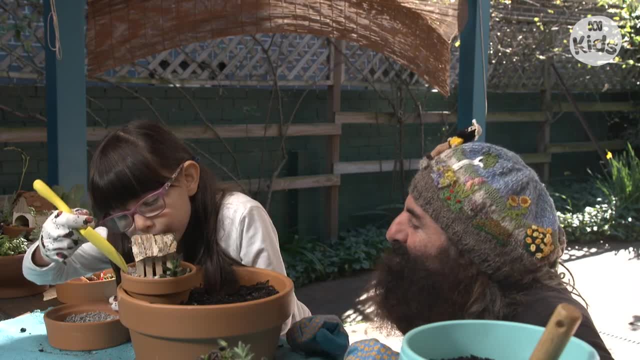 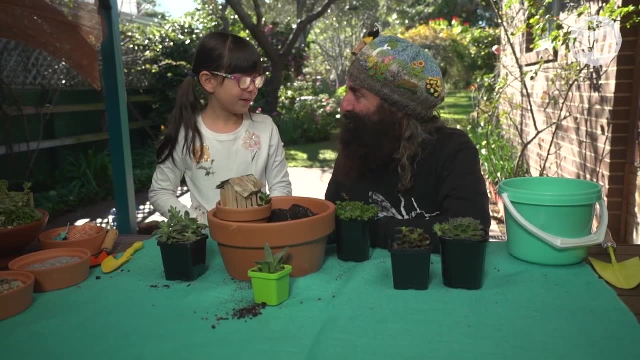 You sort of have to imagine that you're that size, don't you, Mm-hmm, That you're part of this. But what's going to go in this gap? Well, I've got an idea. Ooh, what sort of an idea. 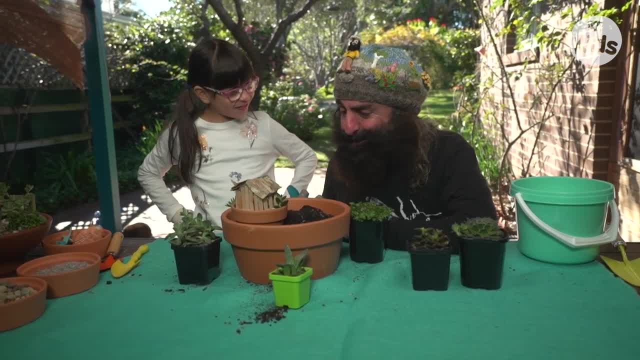 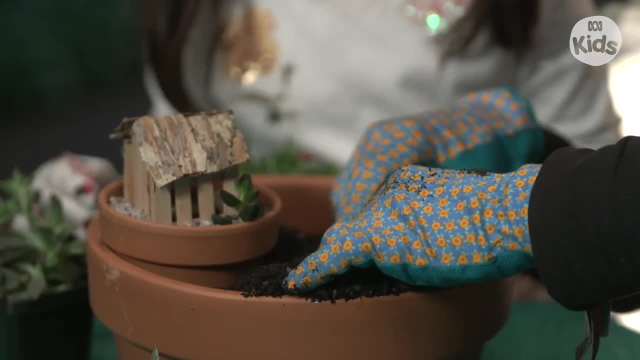 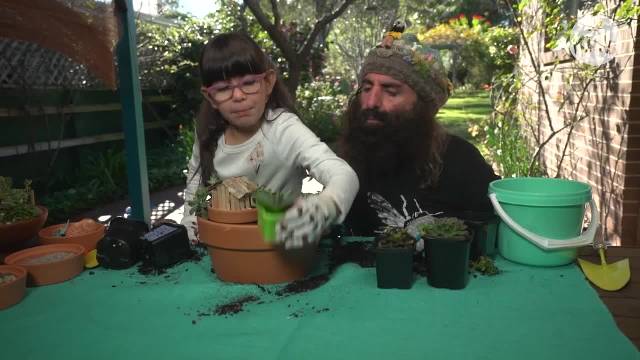 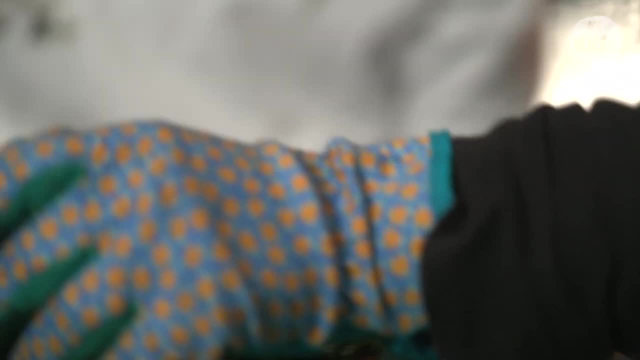 Hasn't it? changed it? Now let's add my small greeny pot. Knock, knock, Who's there? Plants, Plant roots- Here we go. look at that. Now let's build a bridge right here. so it's a little ramp. 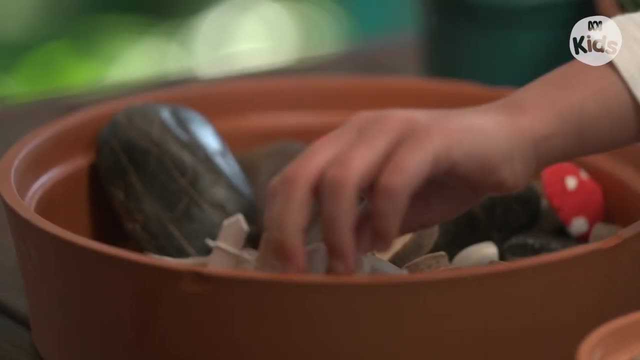 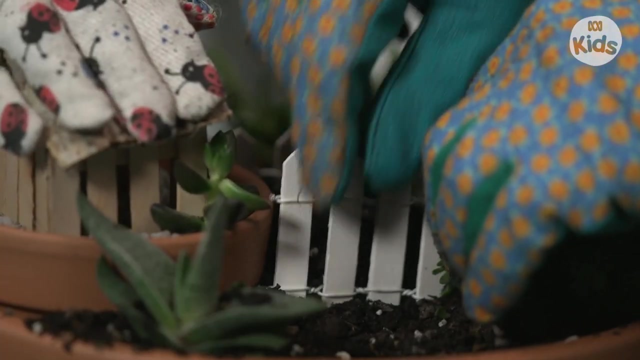 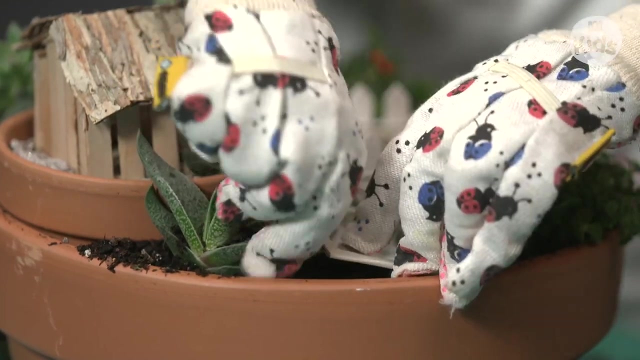 so they don't have to climb, climb, climb A little ramp, yeah, Yes, And then I'll put that up there. So a little bit of Now. let's put this mirror in, And you might be wondering why I'm putting a mirror in. 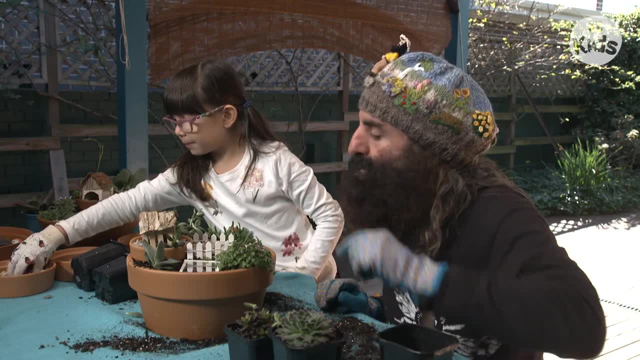 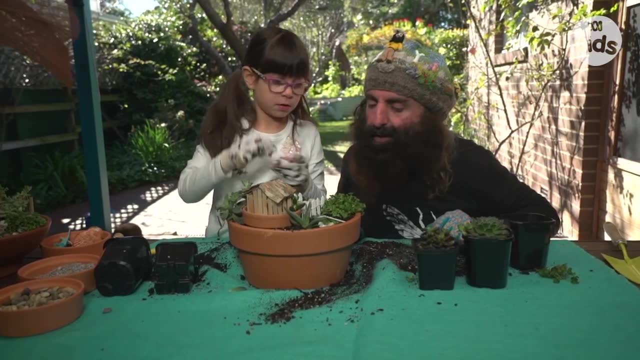 It's going to be a lake, So we're going to cover them up with some stones And that covers the Tape. The edge of the mirror, yeah, Yeah, So you can't see the tape. Yes, Want to help. 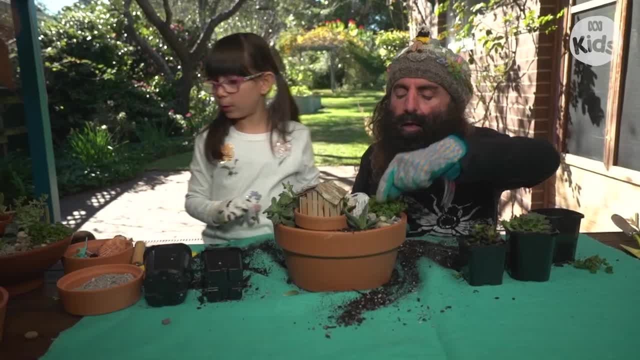 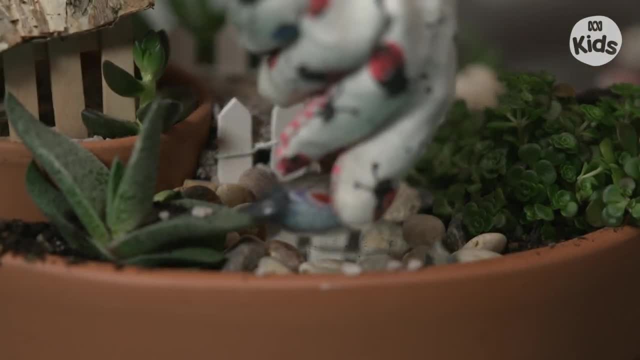 Look at that, And we're going to add some cool animals. Let's see. Oh, what sort of animals do you want to add? Well, we're going to add some baby ducks. It is going to go right here. It's going to sit on the side to look at the babies. 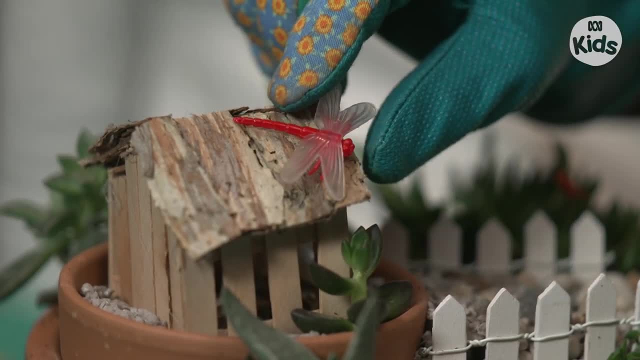 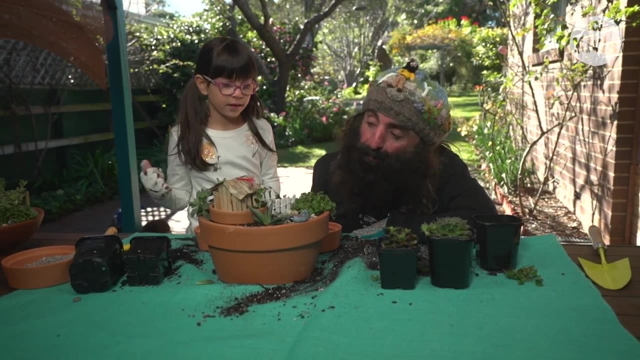 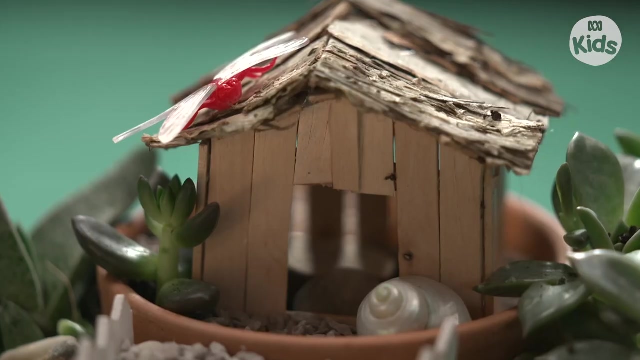 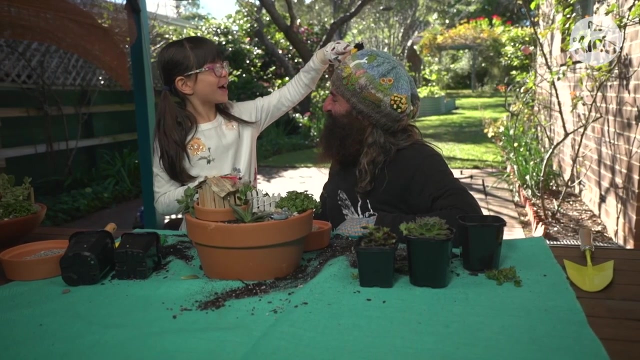 The final touch is a dragonfly. I like it. It just adds that little little touch of red colourness. And this is really showing me up, Is it? And is Mini Costa happy in his garden? Mini Costa, what do you think?